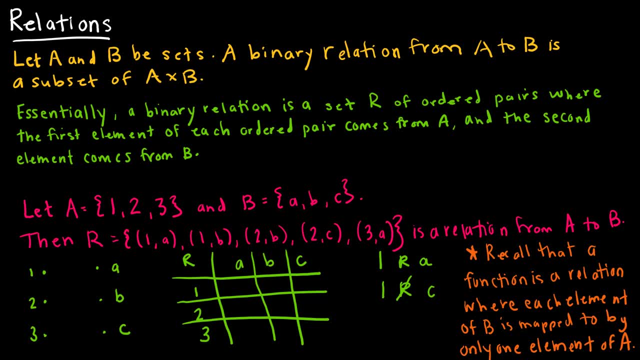 a times b, or essentially, what we're saying is we're going to have ordered pairs where the first value comes from set a and the second value comes from set b. So, for instance, if I have that a is the set containing 1,, 2, 3 and b is the, 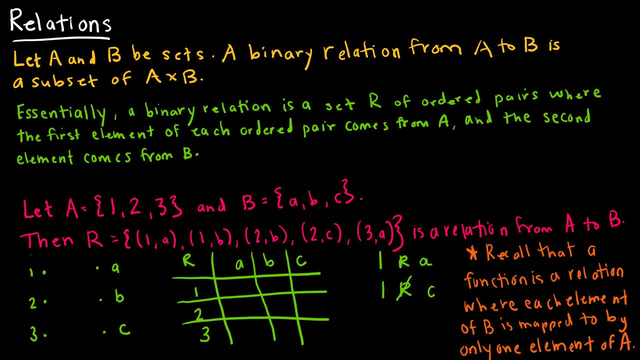 set containing A, B, C. then notice it gives me a relation and the relation includes, in this case, 5 ordered pairs. Now, keep in mind it doesn't include all of the ordered pairs: 1A, 1B, 1C, 2A, 2B, 2C, 3A, 3B, 3C- because it's a subset of A times B, which means it could. 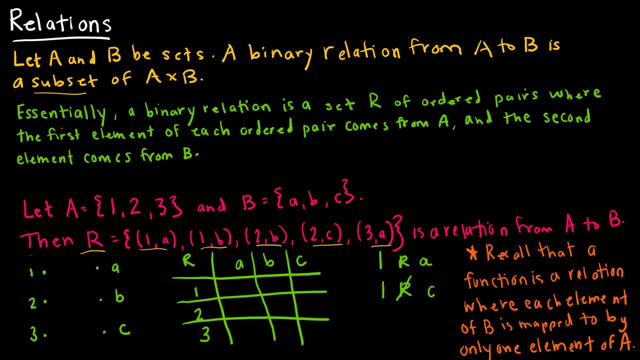 contain all of them, but it doesn't have to. There's different ways that you might see this represented. So we might say that 1 maps to A, that 1 maps to B, that 2 maps to B, 2 maps to C. 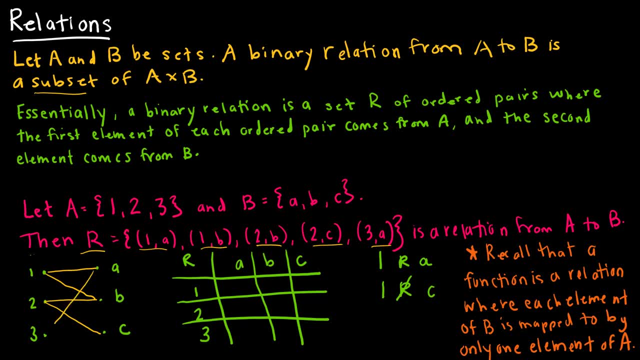 uh 3 maps to A. So that's one way you might see this uh portrayed. We might also see this, where we'll put an X in the table if that value is there. So 1A: yes, we have that in our relation. 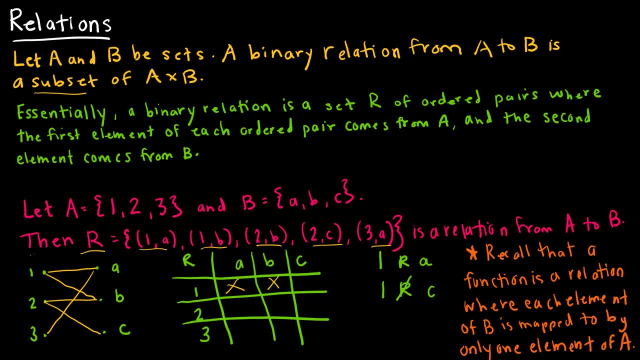 1 comma B: yes, we have that in our relation. 1 comma C: we don't, so we're not going to put an X there. 2A- we do not, but 2A- we do not, So we're not going to put an X there. 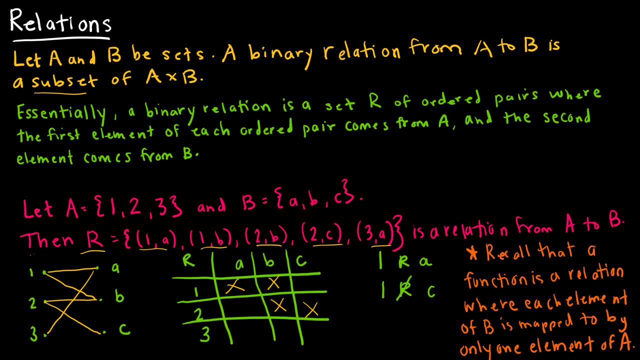 2B we do and 2C we do, and then 3A we do. So again, that's another representation you might see. And then we have 1RA. so that's saying 1 is in the relation with A, but 1 is not. 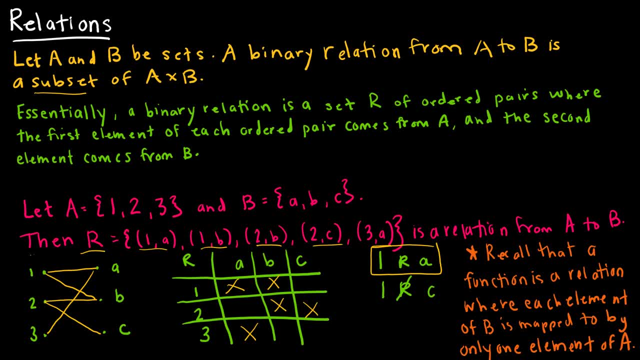 in the relation with, with C, So the relation does not map 1 to C Um, and then recall that if we're dealing with a function, a function is just a special type of relation where every element is a function. So if we're dealing with a function, a function is just a special type of. 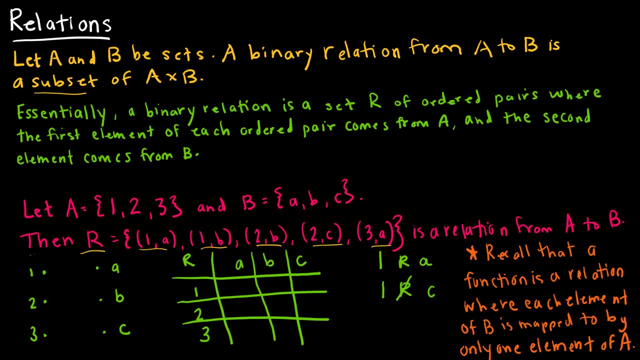 could contain all of them, but it doesn't have to. There's different ways that you might see this represented. So we might say that one maps to a, that one maps to b, that two maps to b, two maps to c, three maps to a. 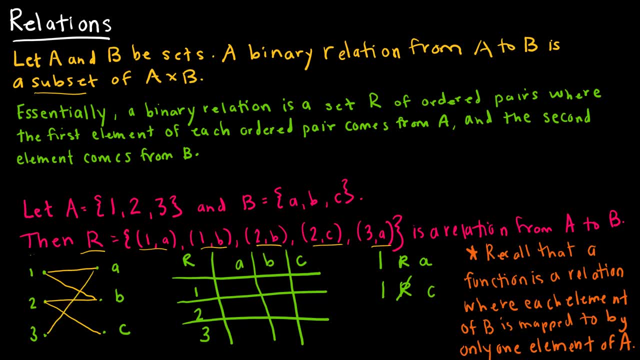 So that's one way you might see this portrayed. We might also see this where we'll put an x in the table if that value is there. So 1a- yes, we have that in our relation 1, b- yes, we have that in our relation 1, c: we don't, so we're not going. 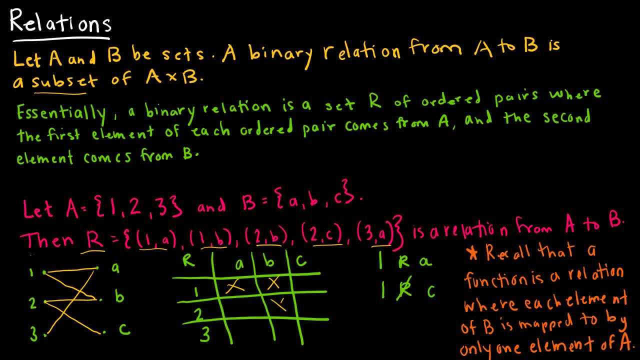 to put an x there: 2a we do not, but 2b we do, And 2c we do, and then 3a we do. So again, that's another representation you might see. And then we have. 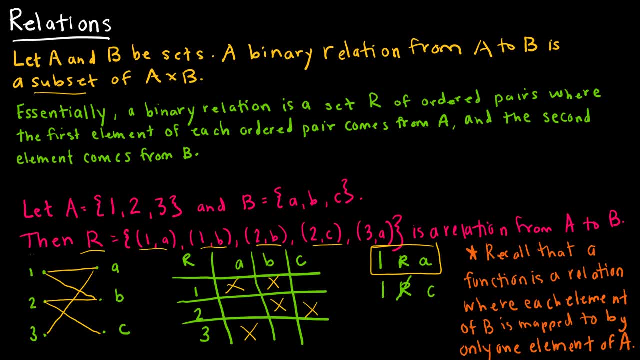 1ra. so that's saying 1 is in the relation with a, but 1 is not in the relation with c. So the relation does not map 1 to c And then recall that if we're dealing with a function. 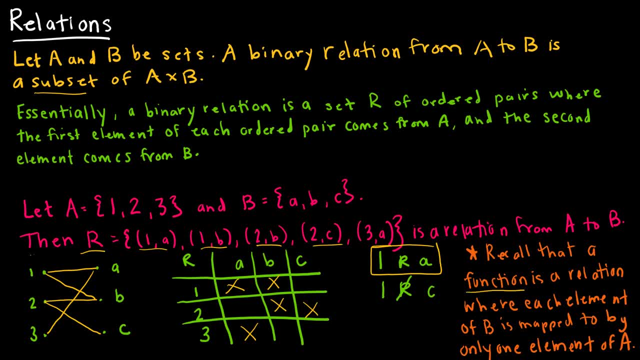 a function is just a special type of relation where every element in b- the second set- is mapped to by only one element of a. So I did not give you an example of that. It's just a reminder that a relation is just a little bit more general because it doesn't have that extra. 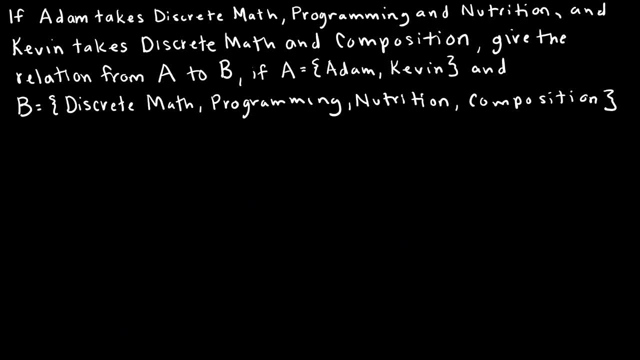 restriction. So if Adam takes discrete math programming and nutrition and Kevin takes discrete math and composition, give the relation from a to b And again a would be Adam, Kevin and b would be discrete math programming, nutrition, composition. So really what we would. 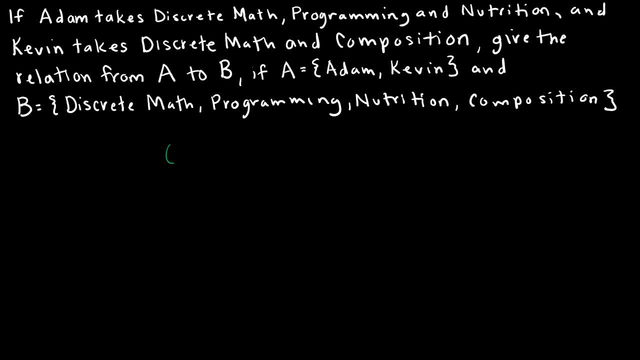 be doing here is just giving all of the ordered pairs. So I should have an ordered pair that maps Adam to discrete, And I should have an ordered pair that maps Adam to programming, And I should have an ordered pair that maps Adam to nutrition. 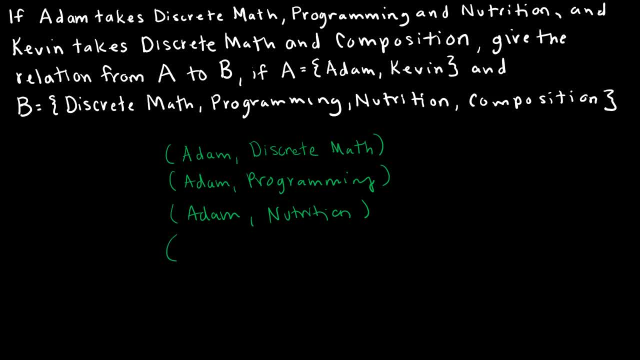 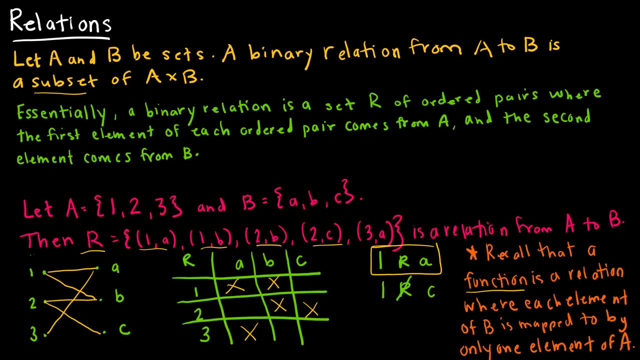 relation. So if we're dealing with a function, a function is just a special type of relation. In B, the second set is mapped to by only one element of A. So I did not give you an example of that. It's just a reminder that a relation is just a little bit more general because it 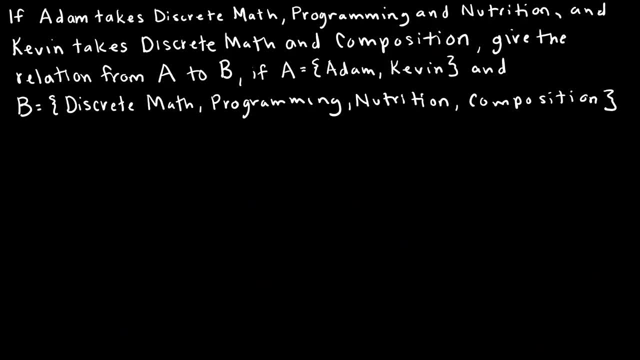 doesn't have that extra restriction. So if Adam takes discrete math programming and nutrition and Kevin takes discrete math and composition, give the relation from A to B And again A would be Adam, Kevin and B would be discrete math programming, nutrition, composition. So really, 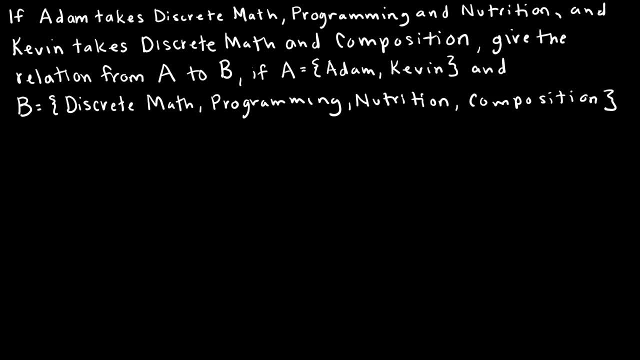 what we would be doing here is we would be adding a function to A and then we would be adding: is just giving all of the ordered pairs. So I should have an ordered pair that maps Adam to discrete, And I should have an ordered pair that maps Adam to programming, And I should have an 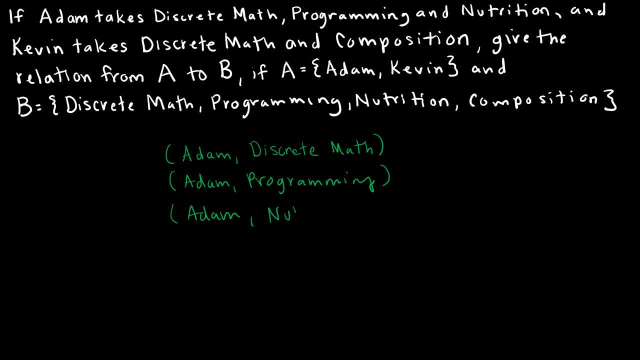 ordered pair that maps Adam to nutrition. I'm sure my brothers love that I use their names in my videos. and then I should. sorry, Eric, I didn't include you on this one. and then Kevin takes discrete. so again, that would be an ordered pair. and then Kevin also takes. 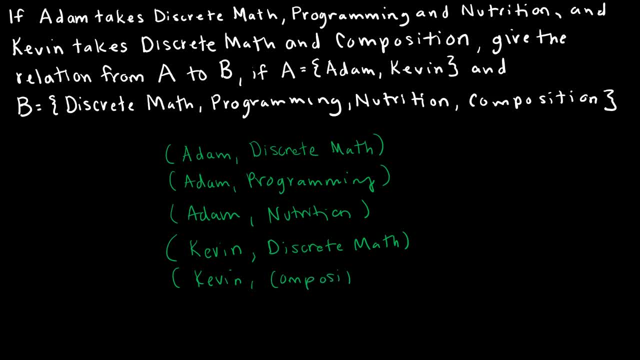 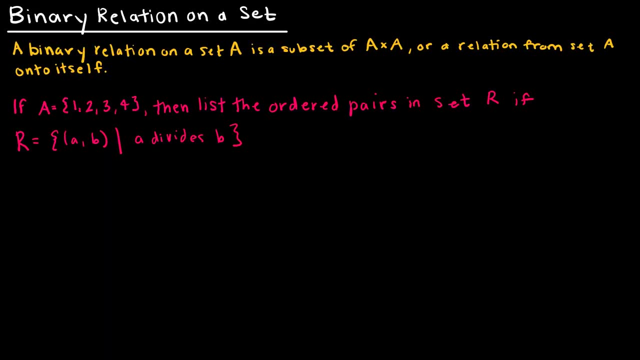 composition. so R would be the set containing all- oops, all- of those ordered pairs. let's take a look now at a relation where I am asking for a relation of a set upon itself. so now I'm just using a twice and notice we have a is four elements and we are going to list the ordered pairs that are in the. 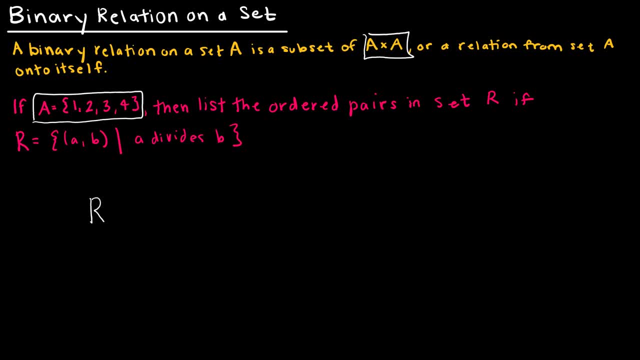 relation or in the set are with this definition. so we're saying the relation is any ordered pairs- a- B- and remember a B have to come from set a, since this is a relation from a to a, where a divides B. so let's remember what it means to say. 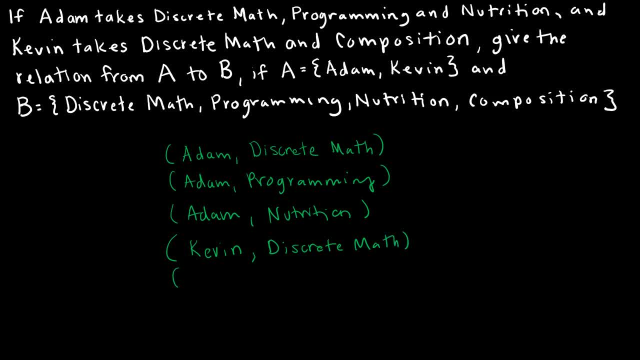 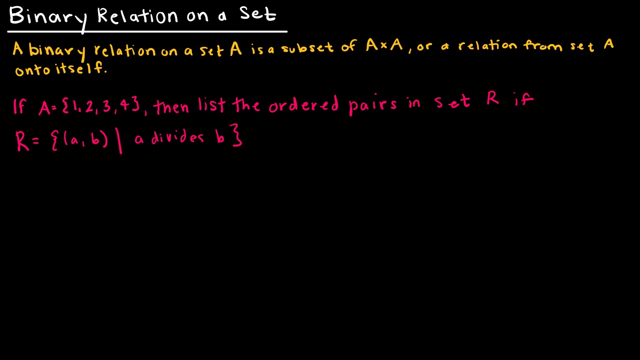 pair, And then Kevin also takes composition, So r would be the set containing all, oops, all of those ordered pairs. Let's take a look now at a relation where I am asking for a relation of a set upon itself. So now I'm just using a twice And notice we have a is four. 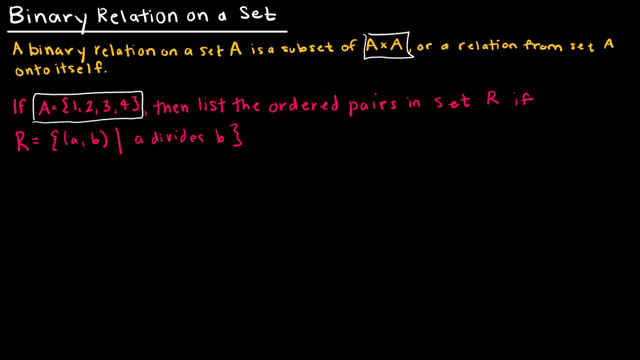 elements And we are going to list the ordered pairs that are in the relation or in the set r with this definition. So we're saying the relation is any ordered pairs- a, b- and remember a, b have to come from set a, since this is a relation from a. 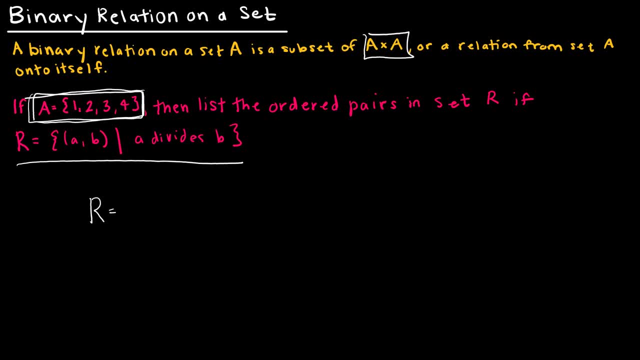 to a where a divides b. So let's remember what it means to say that a divides b. That means that if I took b divided by a, then that solution has to be an integer. So that just means that it has to go into it evenly where there is no remainder. 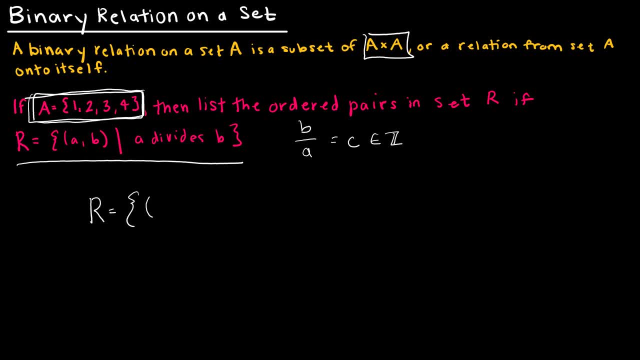 So let's take a look. I should have one comma one because, again, if I took one divided by one, that's a whole number or that's an integer, And if I took two divided by one, that's an integer. So I've got one comma two. Remember: a divides b. 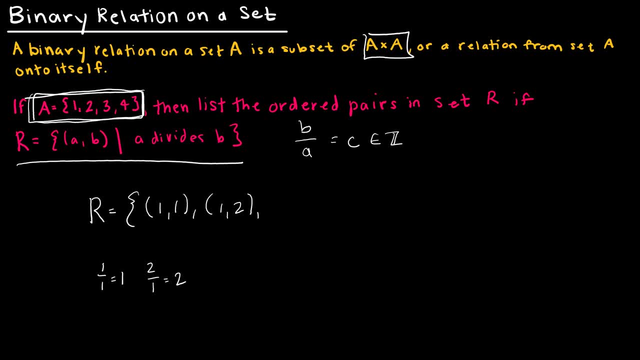 so we have to make sure we're putting this in the proper order. And then three divided by one is three, So one comma three. And then four divided by one is four, So one comma four. So all of those including one or using one as a are in my relation. 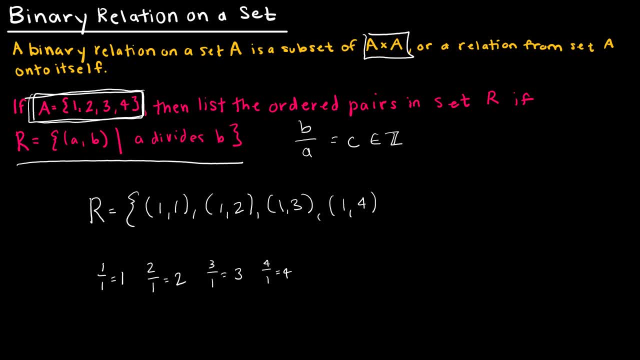 Now let's take a look at two. Could I take one divided by two? No, that's not an integer. take 2 divided by 2?? Yes, that's an integer. So now I have 2, comma 2.. And could I take? 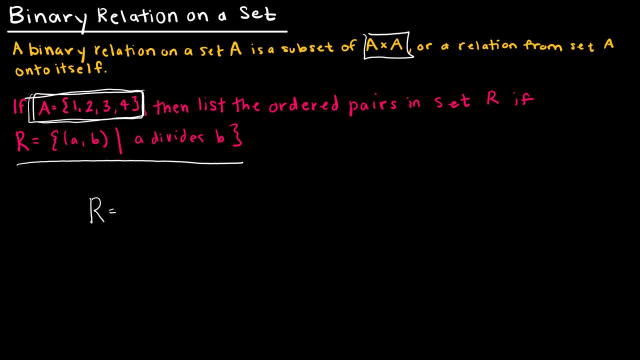 that a divides B. that means that if I took B divided by a, then that solution has to be an integer. so that just means that it has to go into it evenly where there is no remainder. so let's take a look. I should have one comma one. 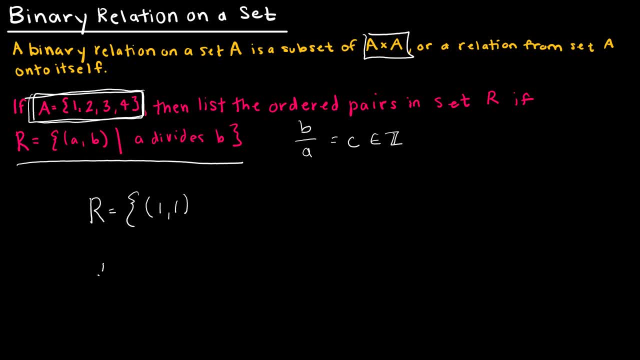 because again, if I took one divided by one, that's a whole number or that's an integer, and if I took two divided by one, that's an integer. so I've got one comma two. remember a divides B. so we have to make sure we're putting this in the proper. 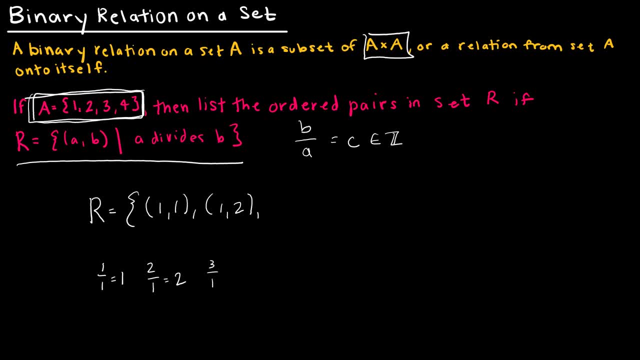 order. and then three divided by one is three, so one comma three. and then four divided by one is four, so one comma four. so all of those, including ones, are using one as a are in my relation. now let's take a look at two. could I take two? 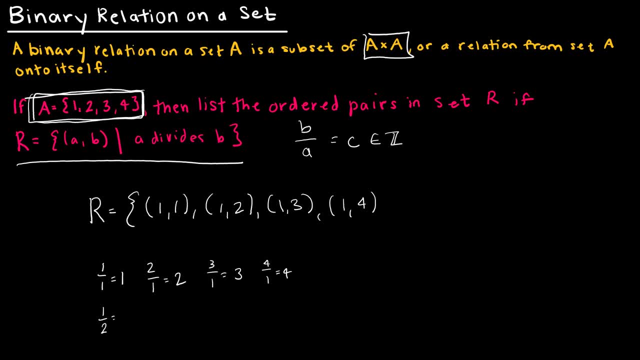 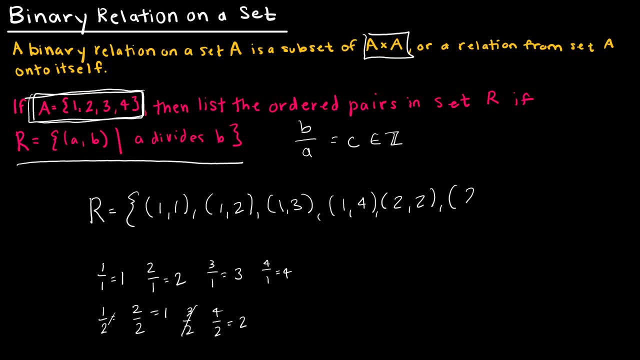 by two. yes, I could. so two comma four. so now let's look at three. could I take three? no, no so, and three comma three. three, I'm going to divide by two. okay, I want to take one divided by three. no, two divided by three. no, three divided by three. yes, 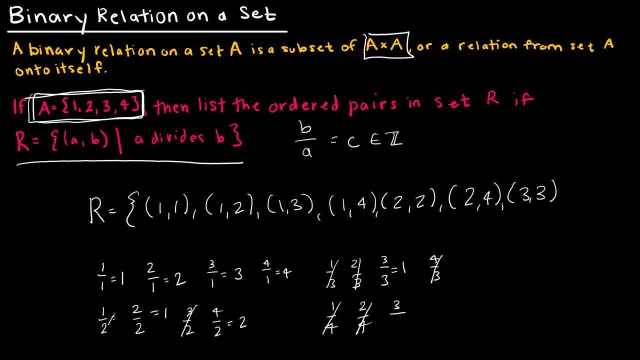 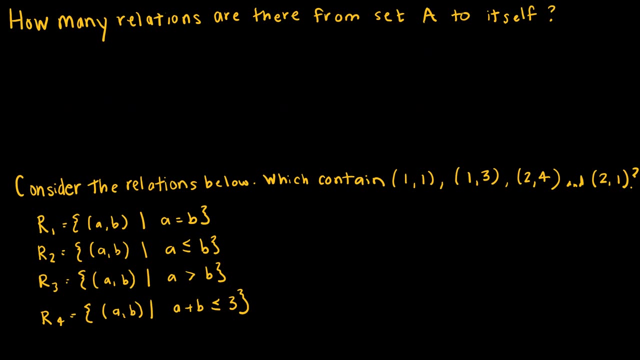 so 33, and then, of course, four divided by three, no, and then I have four. so it could I take one divided by four, no, two divided by four, no. three divided by four, no, but four divided by four is an integer. so this is relation. Let's just look at a couple of practice questions before talking about the properties of. 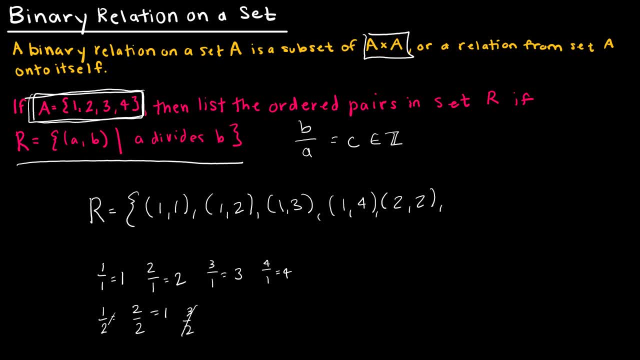 3 divided by 2?? Nope, that's not an integer. Could I take 4 divided by 2? Yes, I could. So 2 comma 4.. So now let's look at 3.. Could I take 1 divided by 3?? No, 2 divided by 3? No 3 divided by 3?. 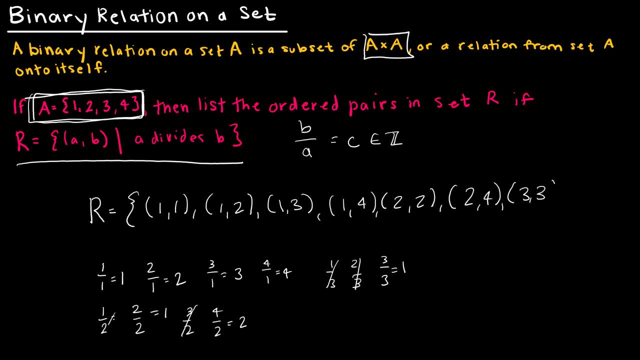 Yes, So 3, 3.. And then, of course, 4 divided by 3? No, And then I have 4.. So could I take 1 divided by 4? No, 2 divided by 4? No, 3 divided by 4? No, But 4 divided by 4 is an integer. 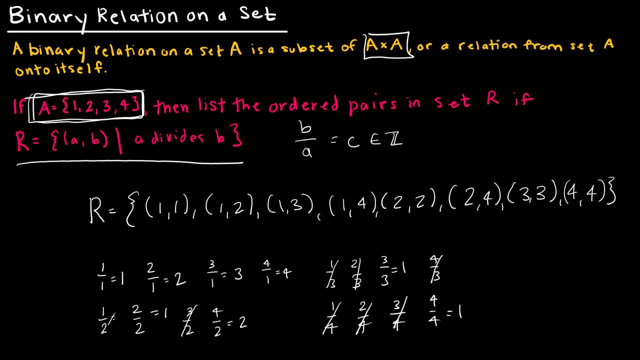 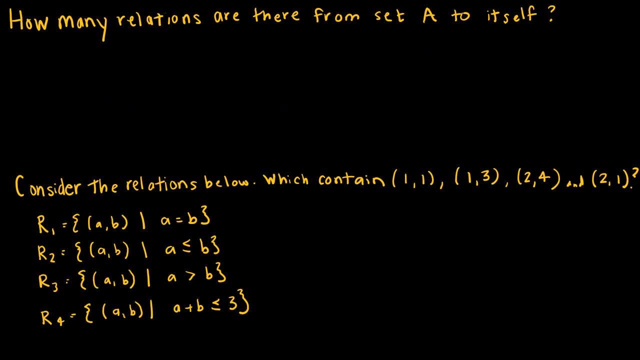 So this is just a listing of all of the elements in that relation. Let's just look at a couple of practice questions before talking about the properties of the property. So let's look at the property of the property. Properties of relations. So first the question asks: how many relations are there from a set A? 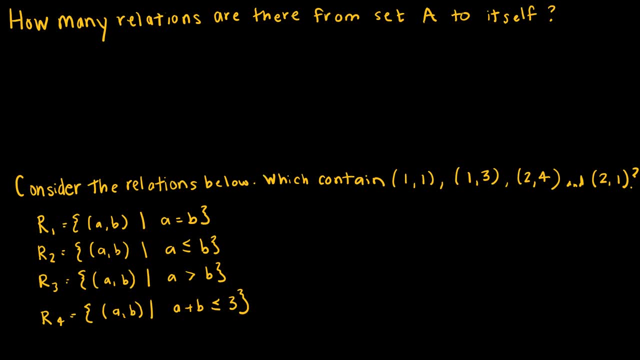 to itself. So let's just assume that set A has n elements. So the cardinality of A is that it has n elements. Remember that a relation is just a subset of A times A, which would mean that this has n elements. So let's just assume that set A has n elements. So let's just assume that set A 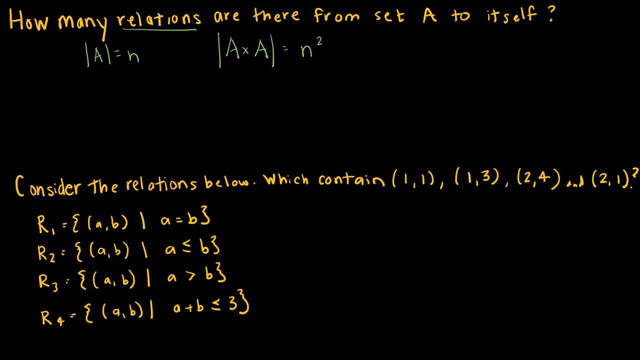 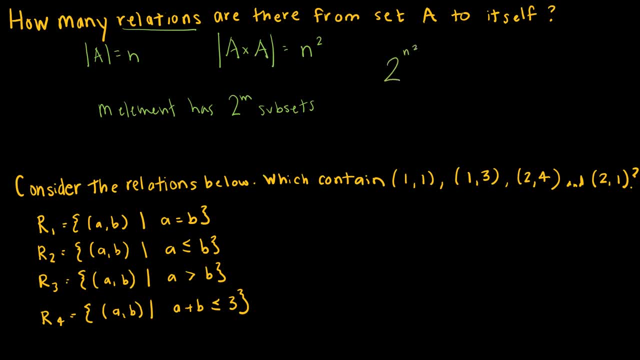 would have 2 to the n squared elements, or you might also see this written as 2 to the cardinality of a squared, which is really the same thing. Now let's look at a little more practical example. We're just asking: hey, here's some relations. 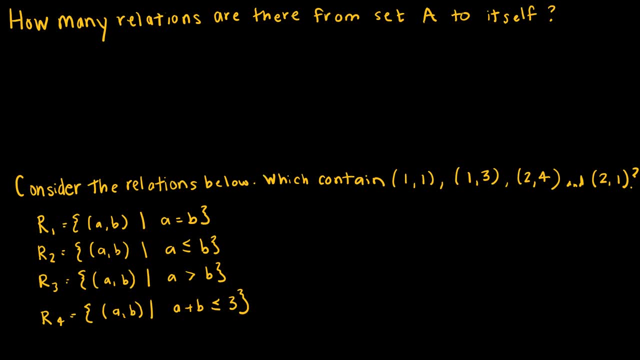 relations. So first, the question asks: how many relations are there from a set A to itself? So let's just assume that set A has n elements. So the cardinality of A is that it has n elements. Remember that a relation is just a subset of A times A, which would mean that this has 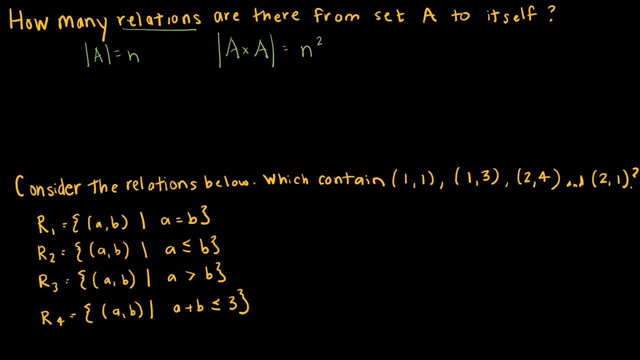 n squared possible. Now we know that a set with m elements has 2 to the m subsets. We learned that a while ago Because, again, each element is either in the set or not in the set and there are m elements. So 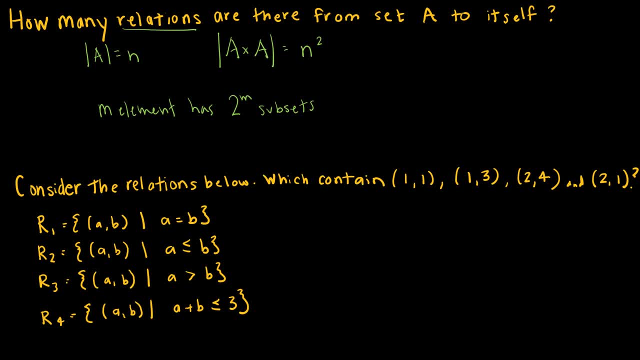 in this case, we can say that a relation from set A to itself would have 2 to the n squared elements, or you might also see this written as 2 to the cardinality of A squared, which is really the same thing. Now let's look at a little more practical. 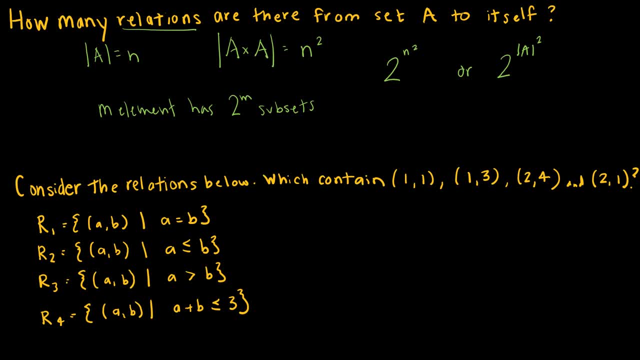 example. So let's say that we have a set A to itself and we have n elements. So let's just confuse the set and say that, for example, we're just asking: hey, here's some relations: 1,, 2,, 3 And 4,. 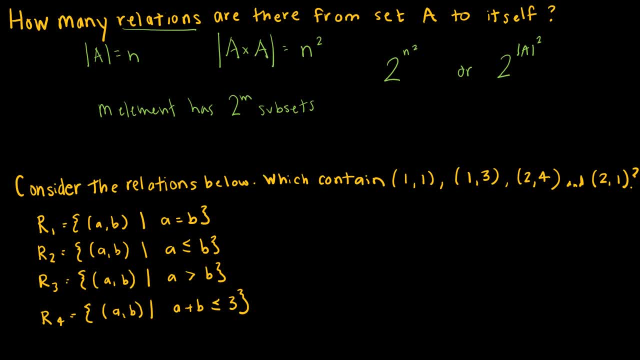 which relations contain the ordered pairs that I have given you. So if I have a relation, umg one that says a comma b, given that a equals B. So looking at my 4 ordered pairs, I can see that one one would be included in that relations. 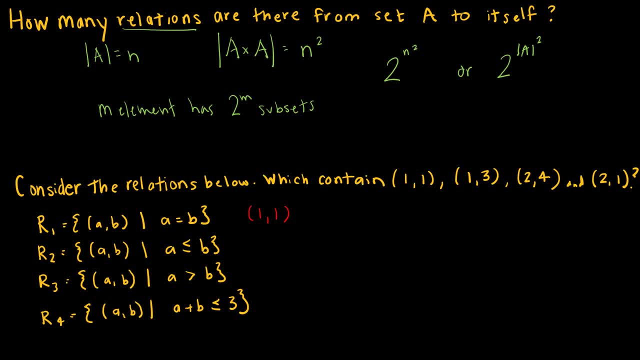 But that the others would not, because none of the other x and y values equal one another For R2,. R2 contains the ordered pairs A- B, such that A is less than or equal to, Less than or equal to. so that means 1 would be included or 1, 1 would be included because 1 is equal to 1.. 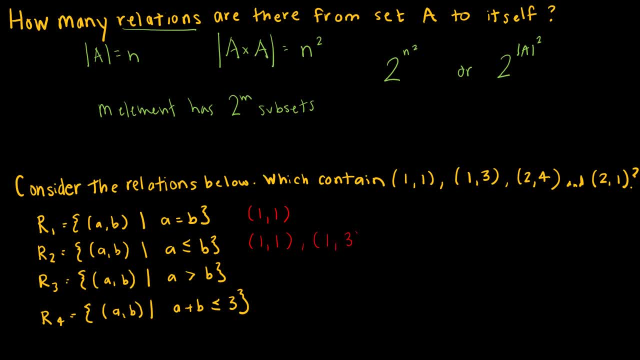 1, 3 would be included, because 1 is less than 3.. 2, 4 would be included because 2 is less than 4, but 2, 1 would not be included because 2 is not less than 1.. 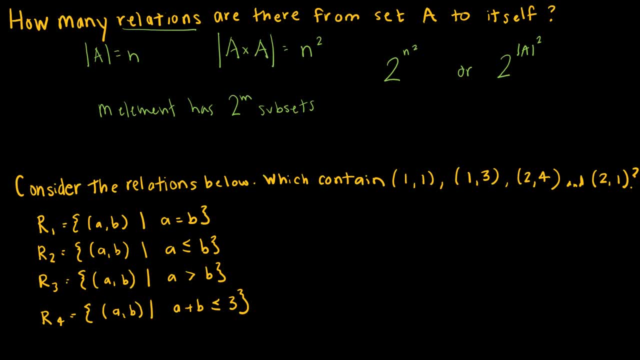 1,, 2,, 3, and 4.. Which relations contain the ordered pairs that I have given you? So if I have a relation 1, that says a comma b, given that a equals b. so looking at my 4, 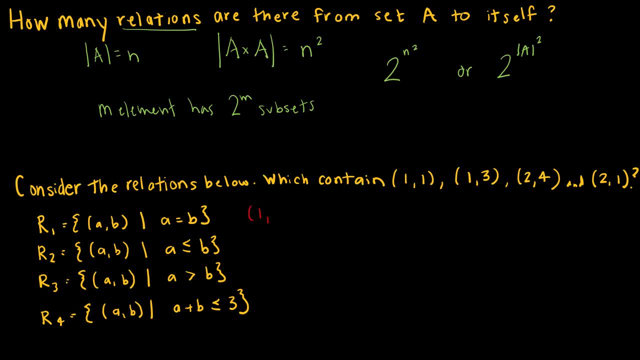 ordered pairs. I can see that 1, 1 would be included in that relation, but that the others would not, because none of the other x and y values equal one another For r2,. r2 contains the ordered pairs a- b, such that a is less than b less than or equal. to excuse me, 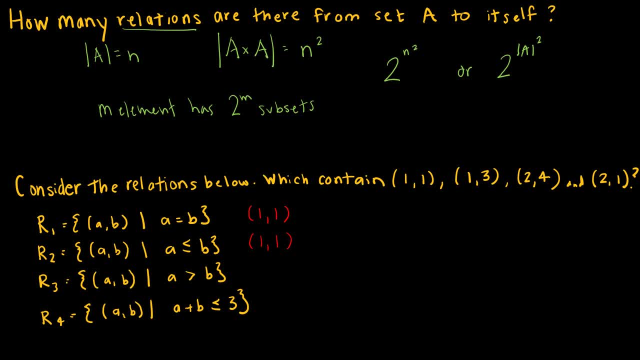 Less than or equal to, so that means 1 would be included. 1, 1 would be included because 1 is equal to 1.. 1, 3 would be included because 1 is less than 3.. 2, 4 would be included because 2 is less than 4, but 2, 1 would not be included because 2 is not less than 1.. 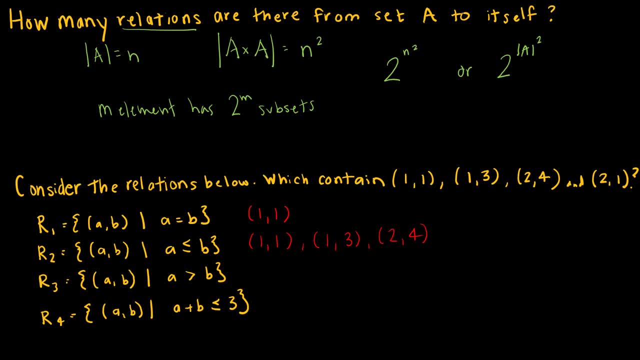 For R3,. R3 contains all of the ordered pairs A- B, such that A is greater than B, and that would be not 1, 1, and not 1, 3, and not 2, 4,, but it would include 2, 1, that lonely little guy we left out last time. 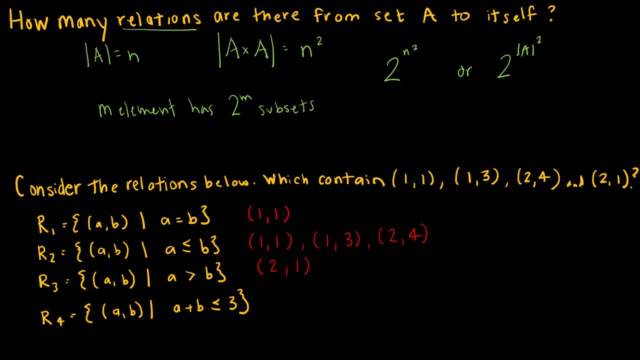 Now, before I look at that last one, I just want to specify- because I didn't before I started the question and I apologize- Notice that I did not tell you, Notice that I did not tell you the values that are in set A and the values that are in set B. 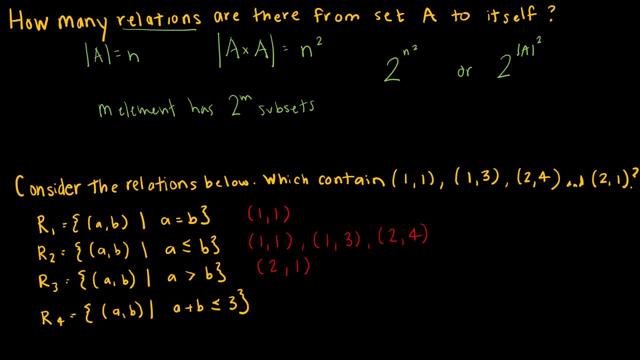 So in this case, I'm looking at the set of A and B, which are infinite sets that contain, you know, all of the integers. Okay, so let's look at R4.. R4 is where A plus B is less than or equal to 3.. 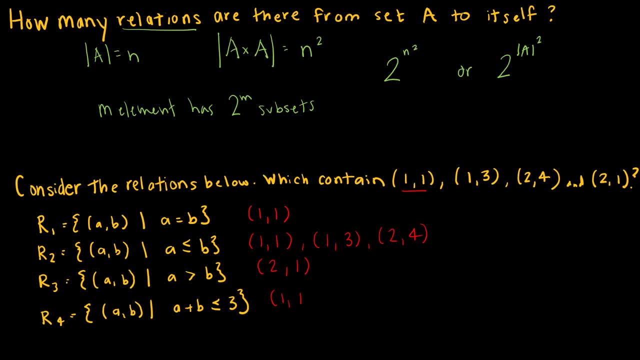 So 1 plus 1 is 2,. that's less than or equal to 3,. so we're good. 1 plus 3,, obviously, is not less than or equal to 3,, so that's good. 2 plus 4 is not less than or equal to 3.. 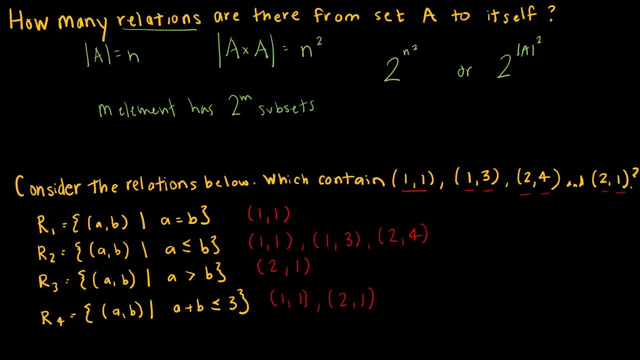 2 plus 1 is 3, and that works. because of that, or equal to Up next, we're going to explore some properties of relations.